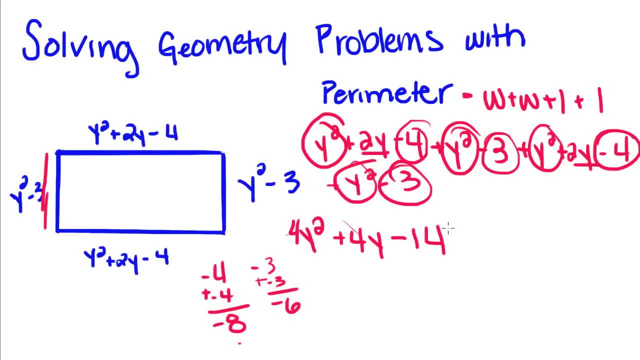 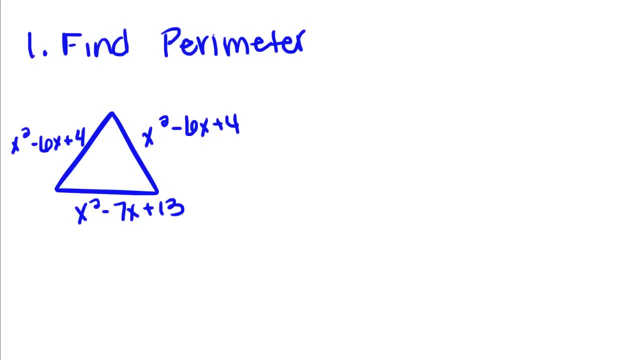 negative. 8 plus negative 6 is negative 14.. So this polynomial right here tells us what the perimeter of this shape is in terms of y. So now we're going to do another example. So for any shape, the perimeter, the way we find the perimeter, is the same. 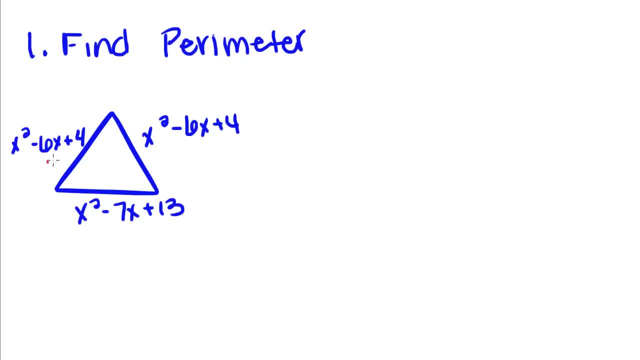 So we're still going to add up each one of these sides and combine our like terms, So x squared minus 6x plus 4 plus x squared minus 6x plus 4 plus y squared minus 7x- excuse me, x squared minus 7x plus 13.. 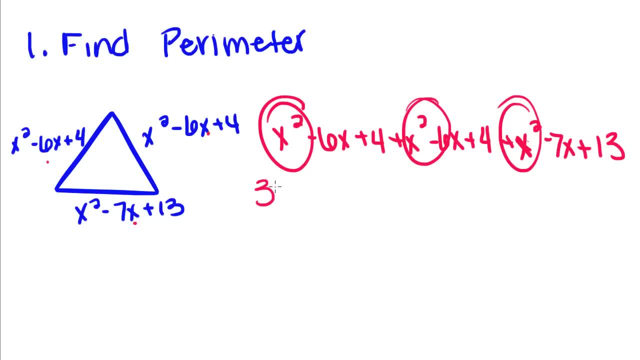 So we're going to combine our x squareds and we have three of them: x squared minus 7x plus 13.. So we're going to combine our x squareds and we have three of them. So we're going to combine our x squareds. negative 6x. negative 6x makes negative 12x. 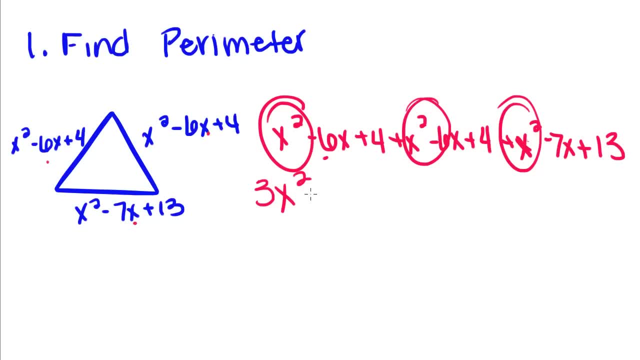 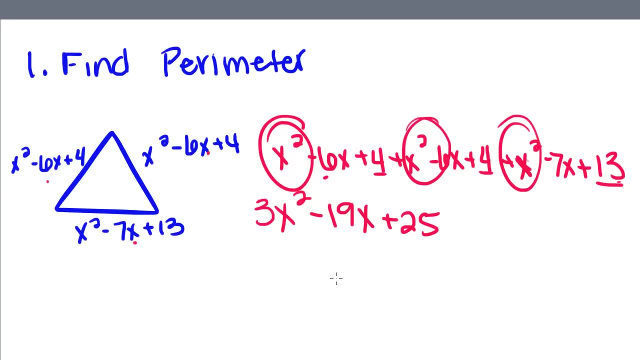 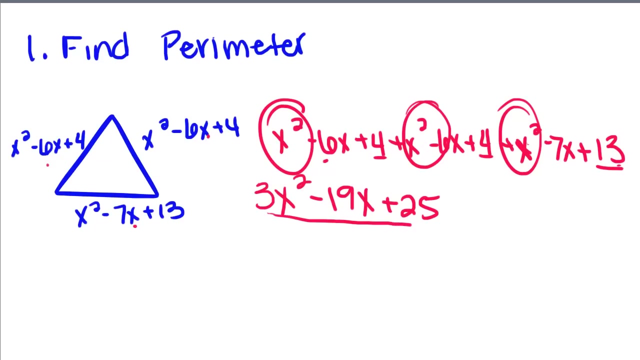 plus negative 7x makes negative 19x, and 4 plus 4 is 8, plus 13 is 25.. So, once again, this polynomial that we ended up with at the end expresses the perimeter of this shape. So now we're going to do the same thing, but with area. 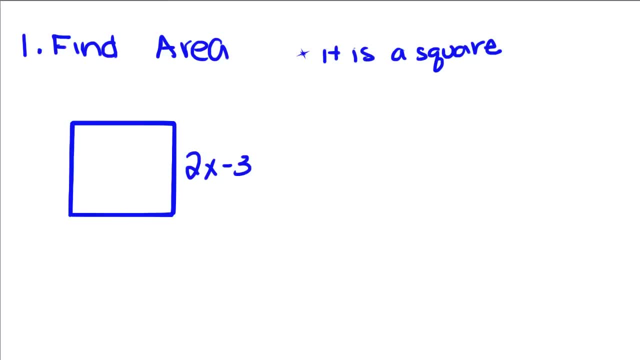 Now, if you remember, the formula for area of a rectangle is length times width. Well, this little note right here that says it is a square, lets us know the area of a square formula which is a side squared, So if we want to know whose side it is right. 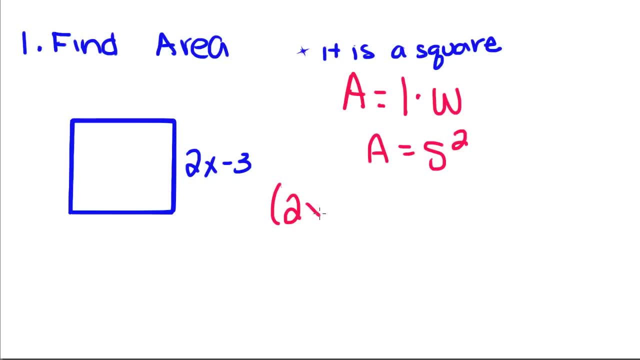 Because this is the litter, this structure of this square, Much easier to understand. So we have to square out this binomial in order to get our area polynomial. So remember, when we square binomials, we write it as two binomials and then we FOIL it out. 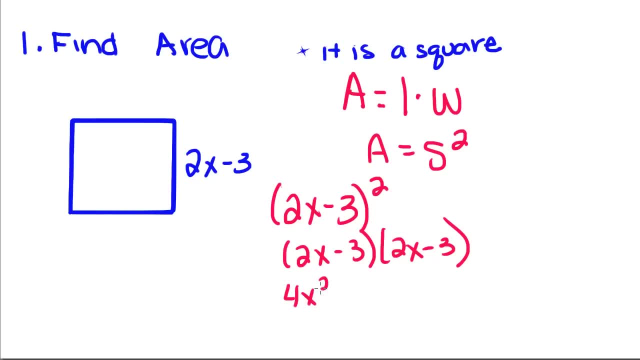 So first is 2x times 2x, which is 4x squared plus outer 2x, minus times negative 3, so negative 6x, negative 3 times 2x. another negative 6x and negative 3 times negative. 3 is positive. 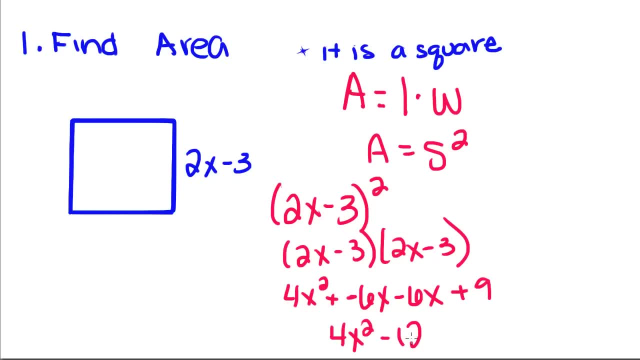 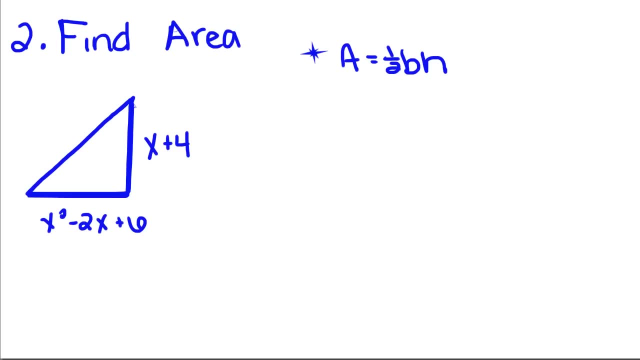 9.. So this is 4x squared minus 12x plus 9.. We're going to do one more example with area Okay, And this time it's with a triangle. So I wrote a little note over here of the area of a triangle, in case you either don't. 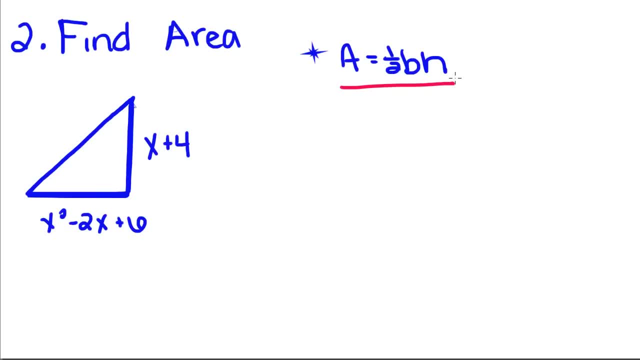 remember from geometry or you haven't taken it yet? So area is equal to 1 half base, which is this one x squared minus 2x plus 6 times the height, which is x plus 4.. And remember, Always use the perpendicular height. 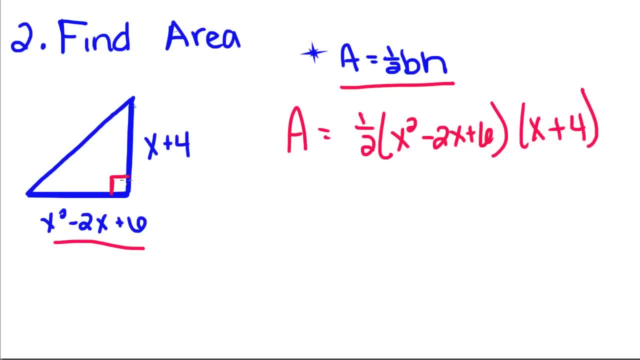 So that has to be right angle right there. So the first thing that we're going to do is distribute this x plus 4 to this polynomial, And then we'll distribute the 1 half later. So 1 half x squared times x is x cubed. 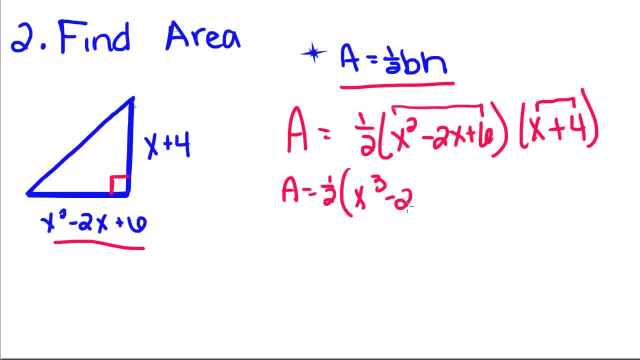 x times negative 2x. So 1 half x squared times x is x cubed x times negative 2x. Negative 2x squared x times 6.. Positive: 6x 4 times x squared. Positive 4x squared. 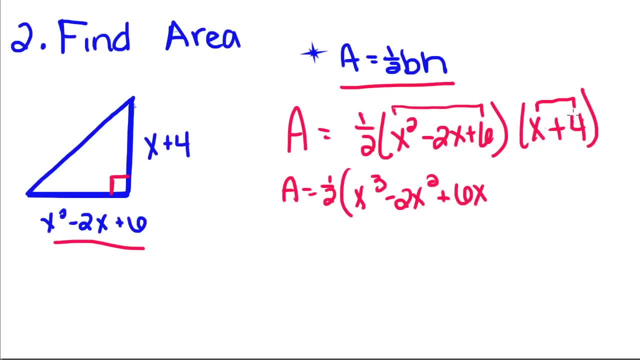 4 times negative. 2x Negative, 8x, 4 times 6. Positive: 24. So now I think it's easier if you combine your like terms first and then distribute this 1 half. So 1 half, we only have 1x cubed. 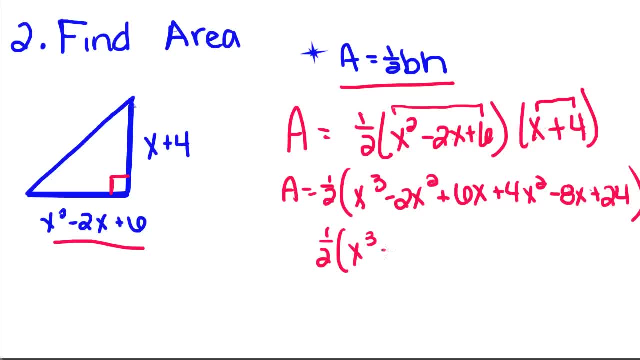 Negative 2x squared plus 4x squared gives you a positive 2x squared, Positive 6x plus negative 8x is going to give us negative 2x And we just have a positive 24 at the end. So now we're going to distribute this 1 half. 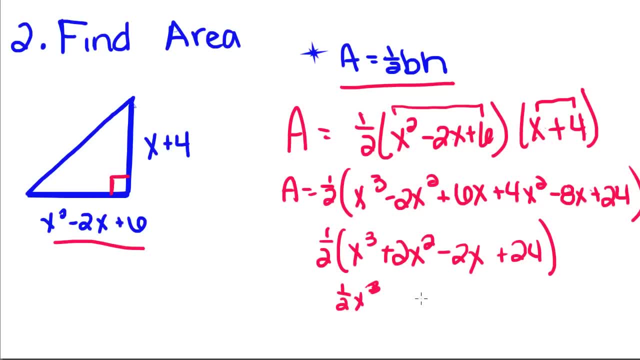 So 1 half x cubed 1 half of 2 is just 1.. So this is x squared: 1 half of negative 2 is negative 1x, And 1 half of 24 is 12.. So that's the area of that triangle.